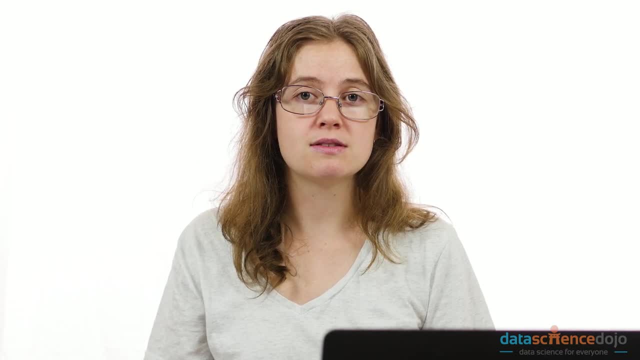 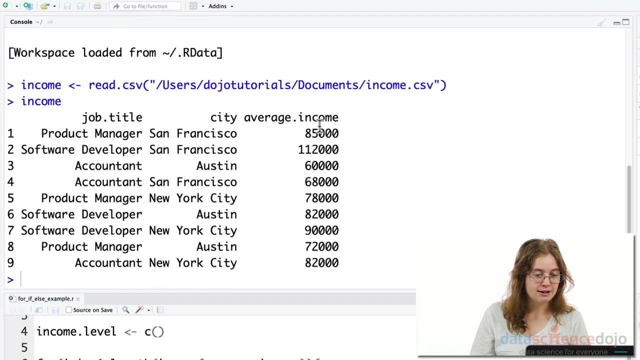 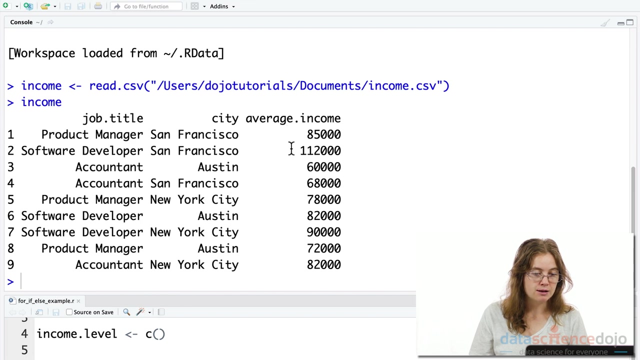 you can learn in programming, but the most useful and simplest control statements are the for loop statement, the if and else statements. So let's just say I have data on the average income for different job roles across, you know, US cities. I want to loop through average income and check if. 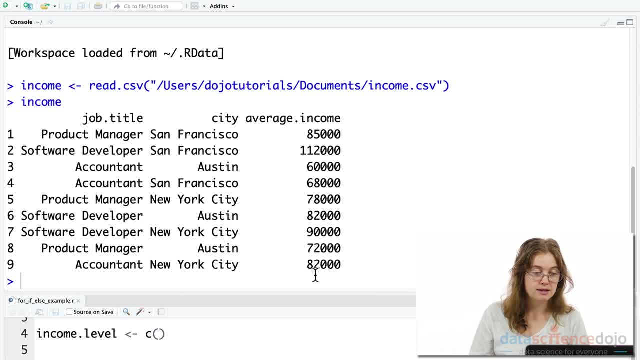 there are incomes greater than or equal to 90,000.. If there are incomes that are 90k plus, I want to tag it as high and store the tag label high in a vector or a list, and for those that fall below this figure they can be tagged low to medium. So to do this and save myself the trouble of 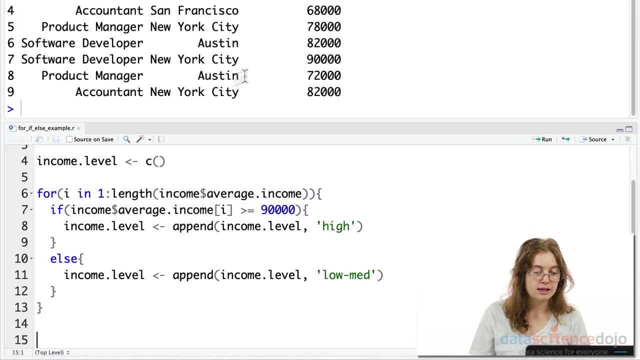 manually checking through the data and tagging it myself. I'll make use of a for loop And an if and else statement. So my for loop will check through each data value in average income, iterating through each value one at a time. My if statement will check if each. 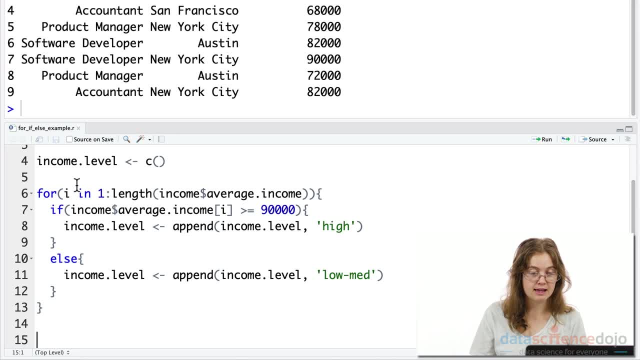 value is greater than or equal to 90k, and if that's the case it'll be labeled high income and stored in a new column vector. Otherwise it will be just labeled as low to medium income. So I have an empty vector tied to a variable called income level, ready for storing the tag. labels high. 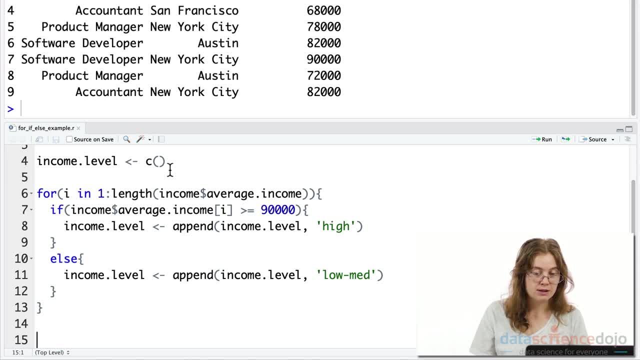 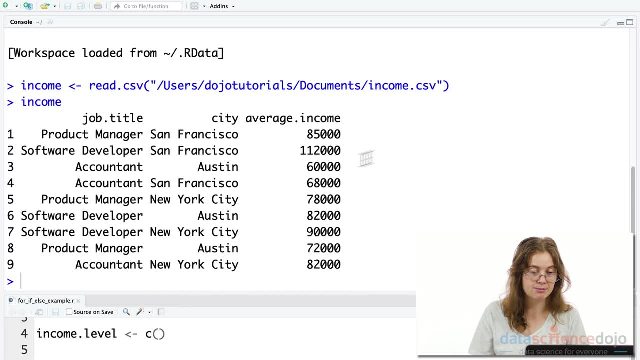 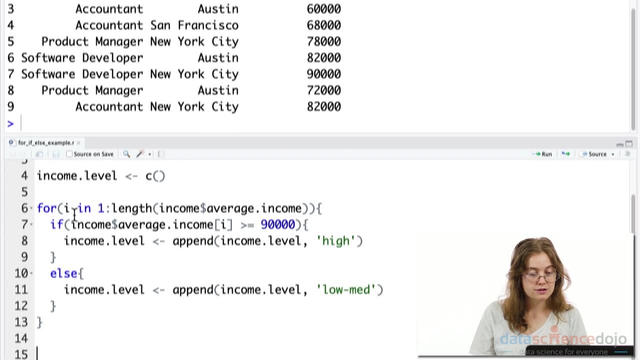 or low to medium in this vector. This is going to be a new column vector that we'll add to our income data later, where the high label corresponds to all cases that are 90k plus and the low med corresponds to all cases that fall below 90k. So then, the way to read this blocker code here is: 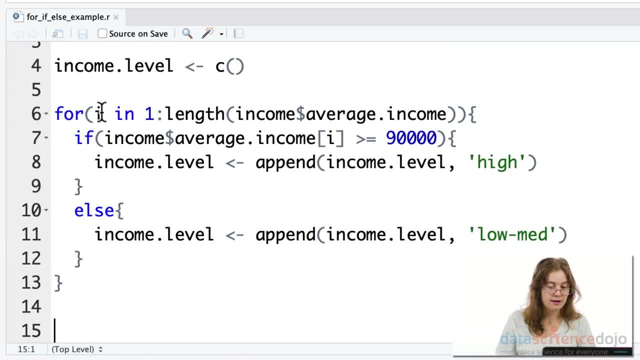 that for each index value, or for i starting at index one, to the last index number, or however long average income is, Check if the income value sitting at that particular index is greater than or equal to 90,000.. If it is, append this onto the end of income level. append the string high. 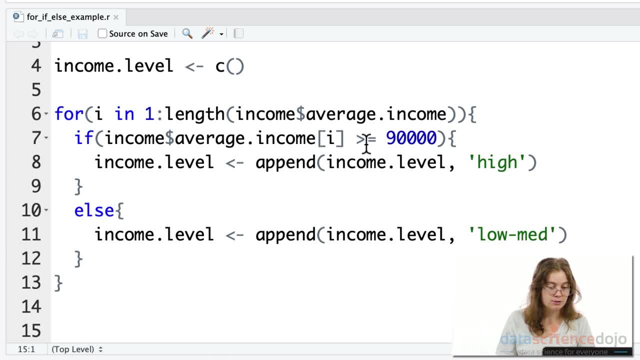 onto the end of income level and keep going through the next value. and if it also meets this condition, append onto the end of income level this, this value, high here, and so on and so forth Else. for everything else that doesn't meet this condition, append the, the value or the string character- low med- onto the end of income level.